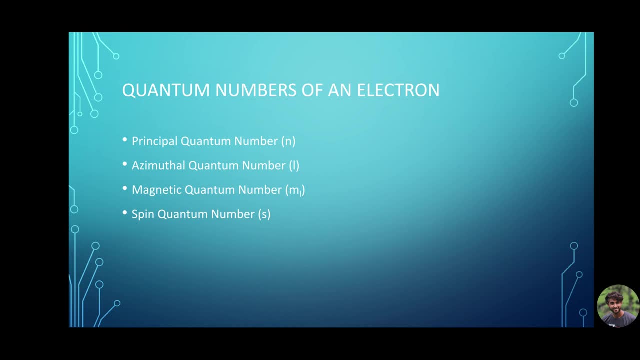 Lowercase n- azimuthal quantum number. lowercase l- magnetic quantum number. lowercase m of l and spin quantum number. lowercase l s. Please note that a quantum description of a molecular orbital require different quantum number, but more of it later. 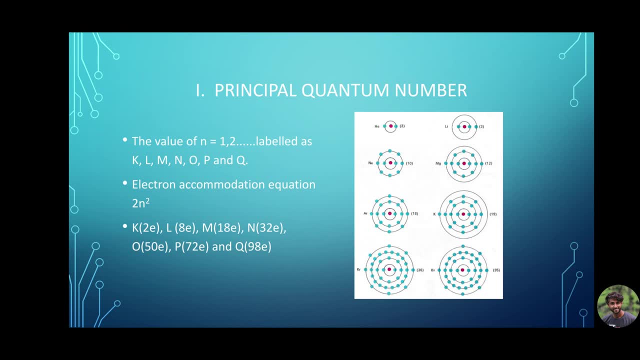 First principal quantum number. This was the first description of an orbital. This was the first description of an atom when we were in junior schooling. An atom has a centralized nucleus and electron revolving around it in orbits, just like solar system. Today we know it is much complex. 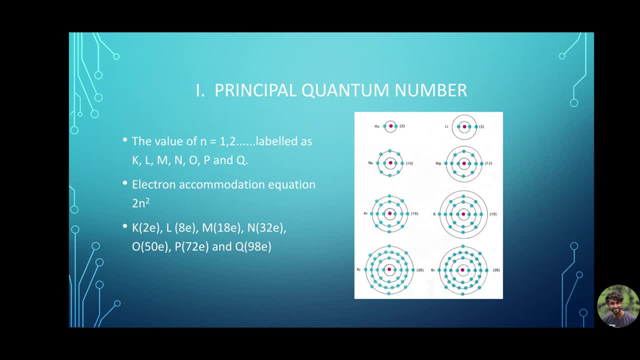 But let us start from there. only This quantum number describe the electron shell or energy level of an electron. The value of n ranges from 1 to 0.. In other words, n is equal to 1 to the shell containing the outermost electron of that. 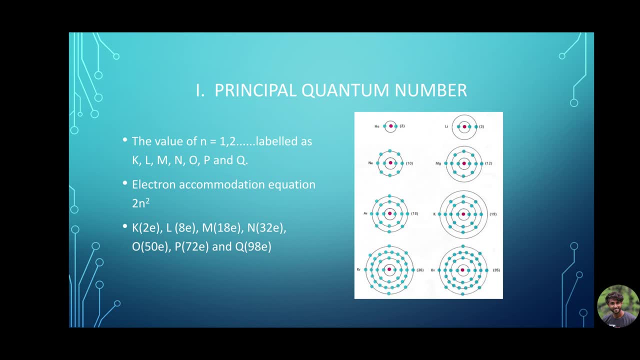 atom, That is, n, is equal to 1,, 2,, 3, etc. The shells are labeled as K, L, M, N, O, P and Q, with electron accommodation described with the equation 2n2.. 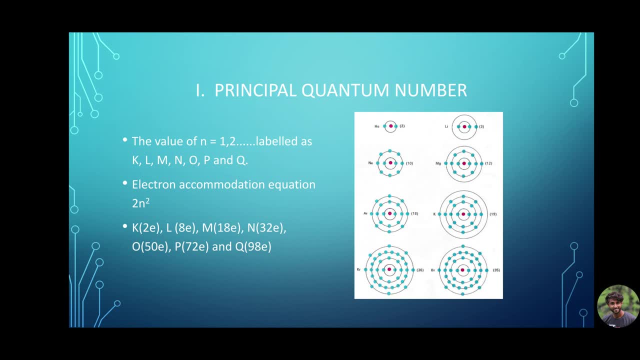 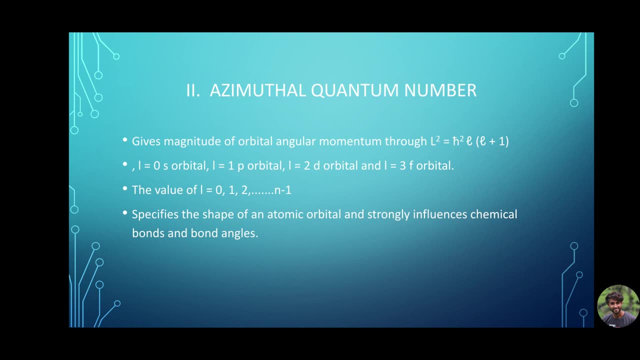 K can accommodate 2 electrons. L can accommodate 8 electrons, Followed by 18 electrons, 18,, 32, and so on. Azimuthal quantum number. Azimuthal quantum number is called the angular quantum number or orbital quantum number. 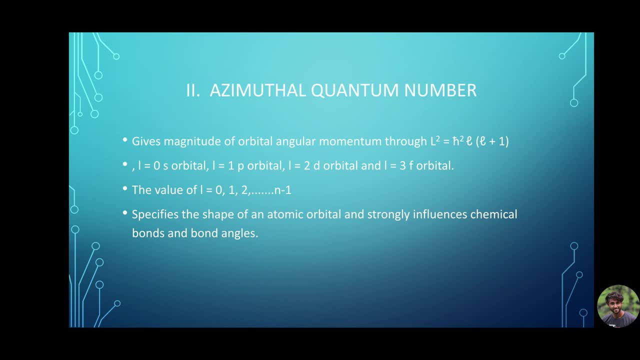 This describes the subshells and gives the magnitude of the orbital angular momentum through the relation: uppercase L square is equal to h bar square of L, of L plus 1, when lowercase L is equal to 0. It is called S orbital. L is equal to 1 is a P orbital. 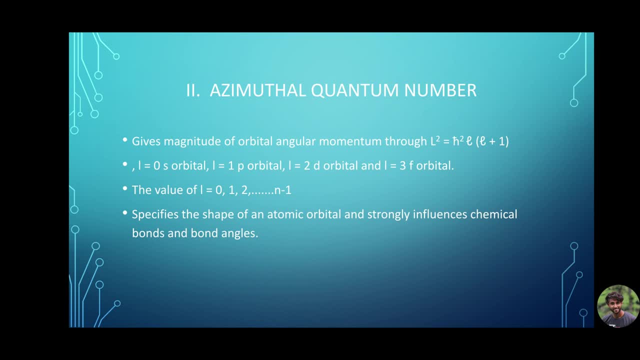 L is equal to 2- a d orbital, and L is equal to 3- an F orbital. The value of L ranges from 0,, 2,, 3, 4 up to n minus 1.. This is an important quantum number as it specifies the shape of an atomic orbital and 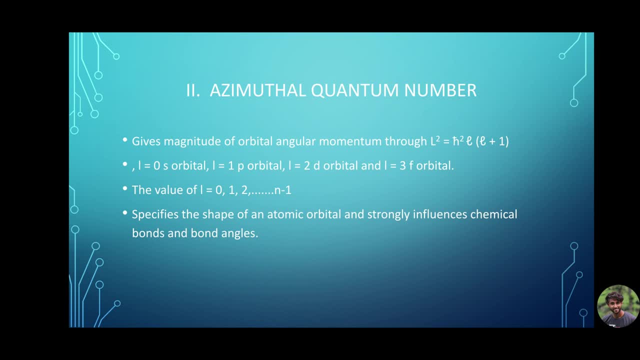 strongly influences chemical bonds and bond impulses. We can now see that the shape of the orbital is the shape of an atomic orbital and not a spawn angles. For example, a quantum number n is equals to 3,, l is equals to 0. describe an. 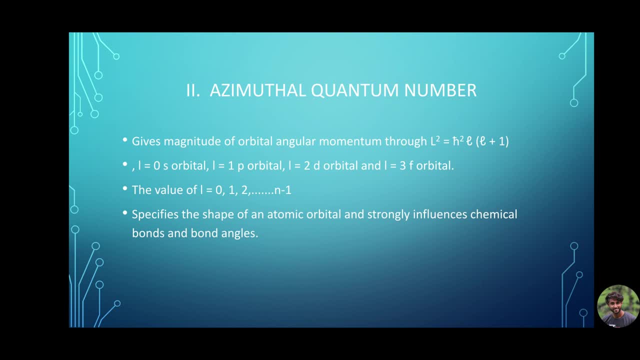 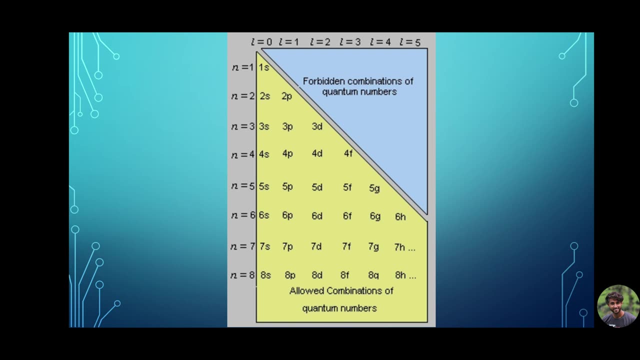 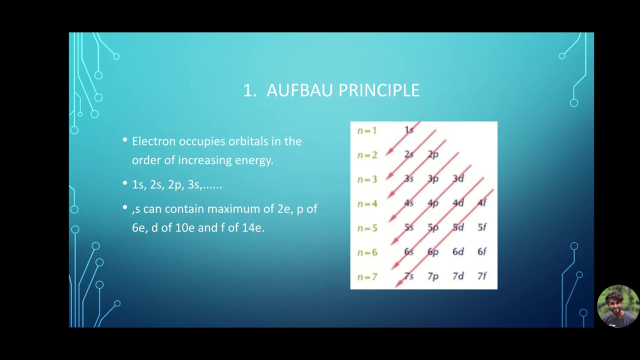 electron in the s orbital of the third electron shell. The diagram here shows the electron orbitals and orbit. Let me add orbital filling rules along the way. Offer principle. Offer is German word for building up. It says that electron occupy orbitals in order of increasing energy, as shown in the slide: First 1s, then 2s, 2p. 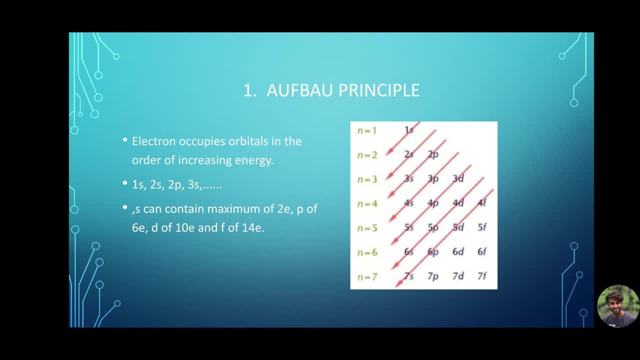 3s and so on. S can contain a maximum of 2 electron, p of 6 electron, d of 10 electron and f of 14 electron. Here 1,, 2, and 3 represent the specificity, which represent the shell number or the principle quantum number. 1s is s-orbital in k-shell. 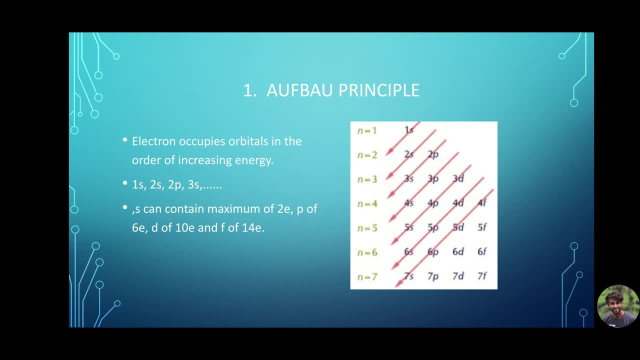 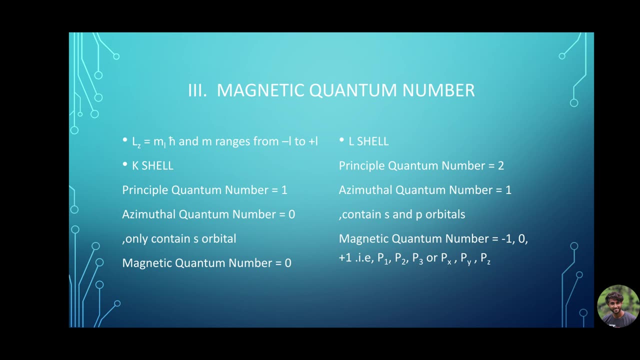 2s, 2p are s and p orbitals in L-shell Magnetic quantum number 23.. ну 2 dimensorsγ. Magnetic quantum number describe the specific orbital within the subshell and yields the projection of the orbital angular momentum along a specific axis. 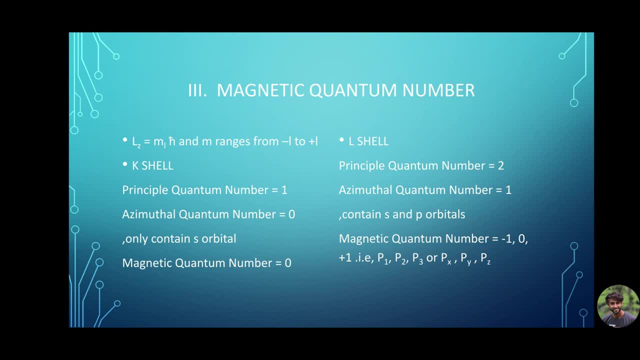 L of z is equals to m of l. h bar Value of m ranges from minus l to plus l. This is where some confusion start and we will clear that According to the quantum number. so far, let us see the first shell, K-shell. 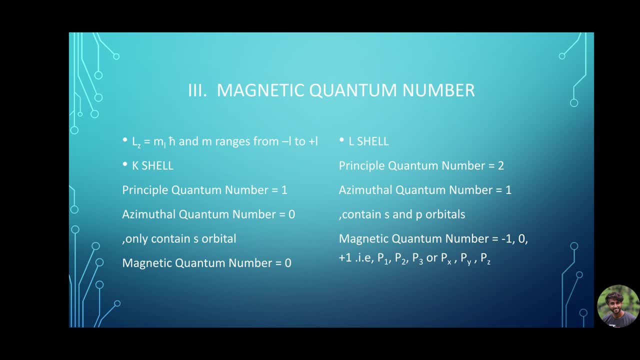 K-shell has principal quantum number 1 and azimuthal quantum number 0.. That is, it only contain s subshell. Here magnetic quantum number is equal to 0.. L-shell: L-shell has principal quantum number 2 and azimuthal quantum number 1.. 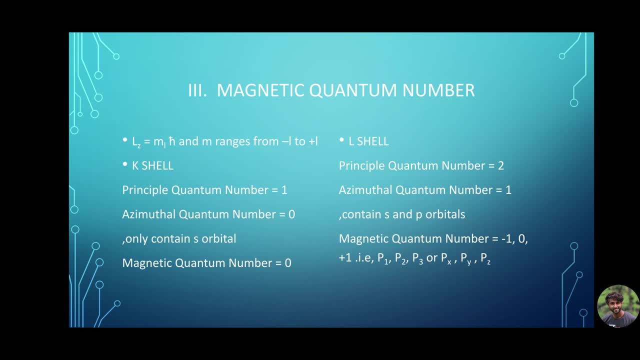 Thus magnetic quantum number is equals to minus 1, 0, plus 1.. Now what does that mean? L has an s orbital with m is equals to 0 and a p orbital with m is equals to minus 1, 0,. 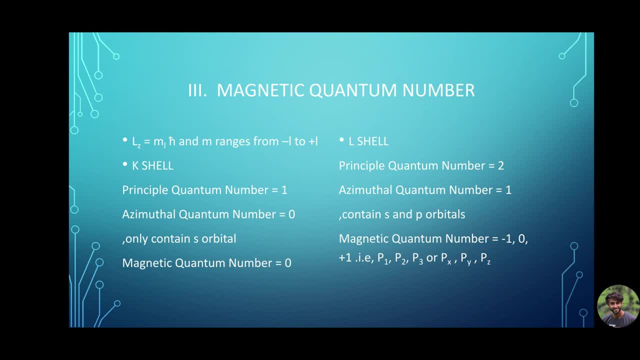 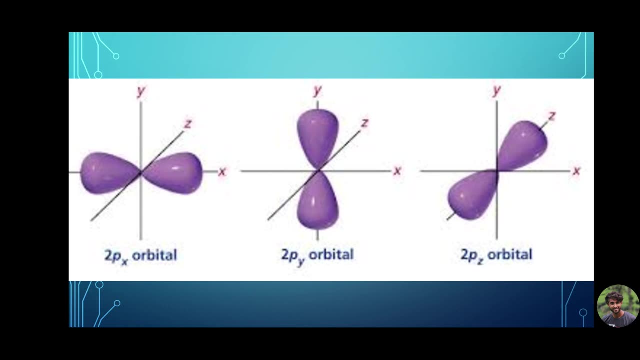 plus 1.. That is px, py, pz or p1, p2, p3.. P orbital are dumbbell shaped In comparison to the spherical s orbital. this is how p orbital looks like. This is the representation of 2px, 2py and 2pz orbitals. 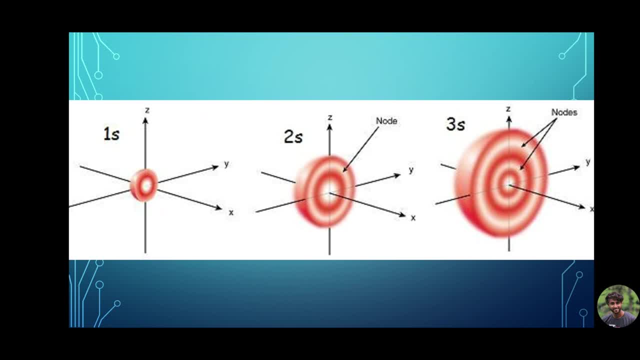 This is how an s orbital looks like. This is the representation of 1s, 2s and 3s s orbitals. The cavity between consecutive s orbital is equal to 0.. The field is called s orbital and the probability of finding the electron in a node is 0. 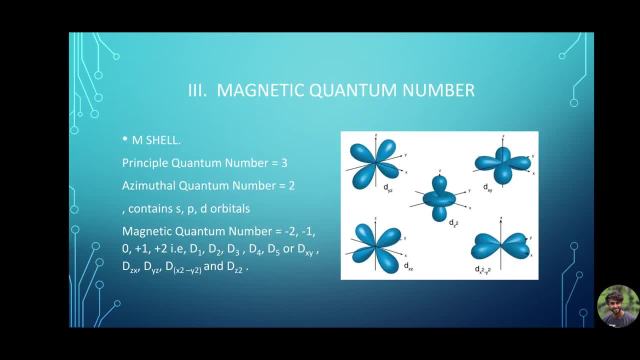 If the conductor is a quantum number, the crystal s orbital is also equal to 0.. So we have a d-orbital Now. this is d-orbital. This is a d-orbital. It contains 2s, 2s and 3s as the particle and the probability of finding electron in 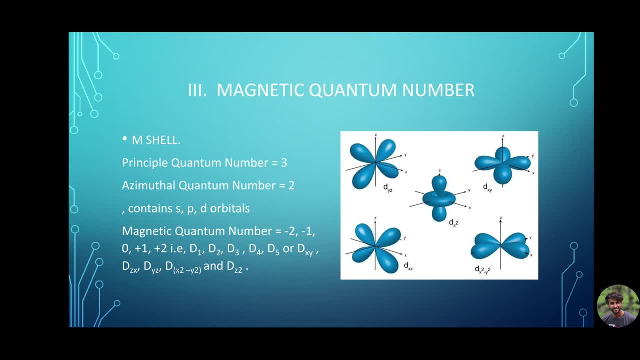 a d-orbital is 0.. The number of channels that contain these electrons is equal to 0.. m-shell has principal quantum number 3, azimuthal quantum number 2,, as it contain d-orbital 1p subshell with px, py, pz. In addition to that, now we have 1d subshell with: 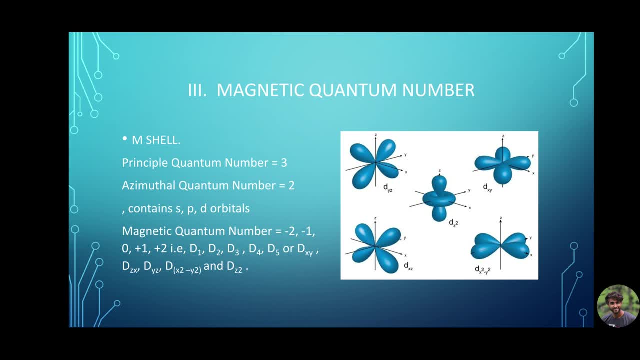 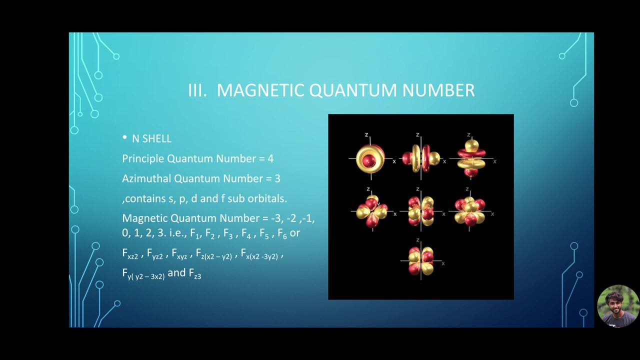 minus 2,, minus 1,, 0, plus 1 and plus 2, or dxy, dzx, dyz, dx square minus y square and dz square. The figure represent the d orbital. Likewise, f subshell has minus 3,. minus 2,. 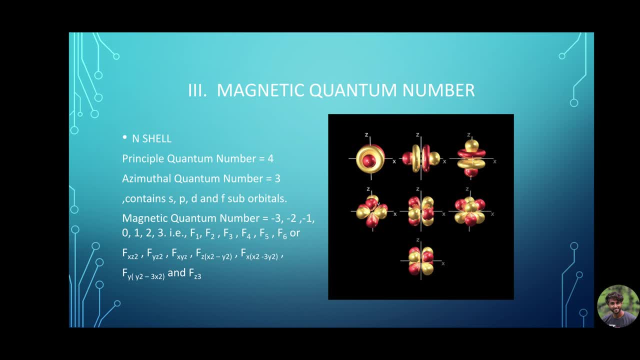 minus 1,, 0,, 1,, 2,, 3.. That is f, f, f, f, f, f, f, x square minus 3y square, fy of y square minus 3x square and f of z square. This is: 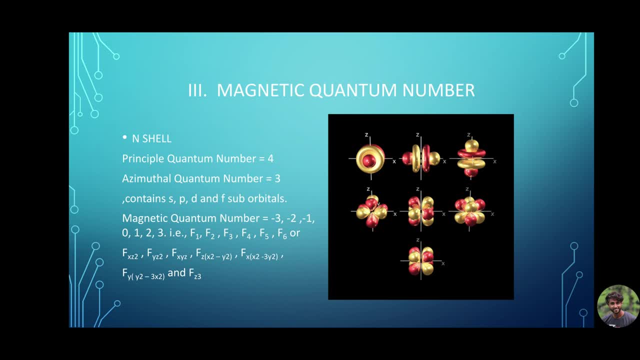 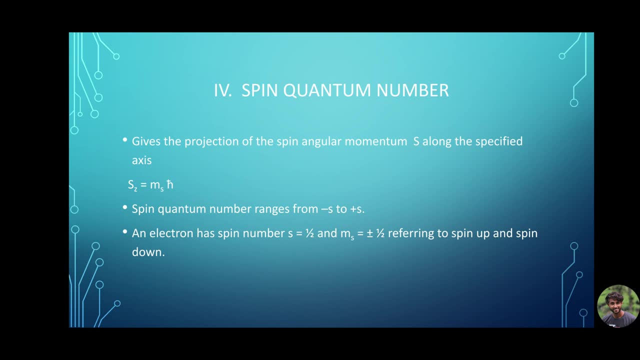 how an f orbital looks like. Next, spin quantum number. Spin quantum number describes the spin of the electron within that orbital. It is an intrinsic angular momentum. It gives the projection of the spin angular momentum along the specific axis. S of z is equals to m of s h bar. In general, the value of 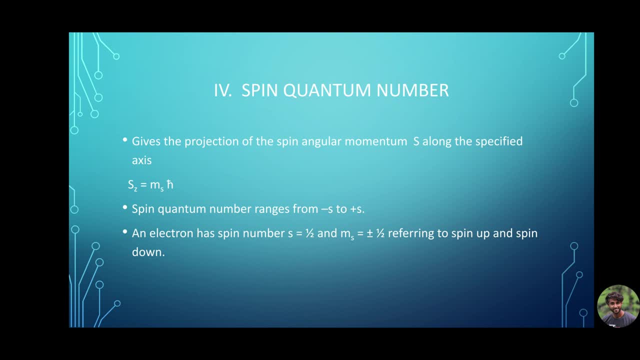 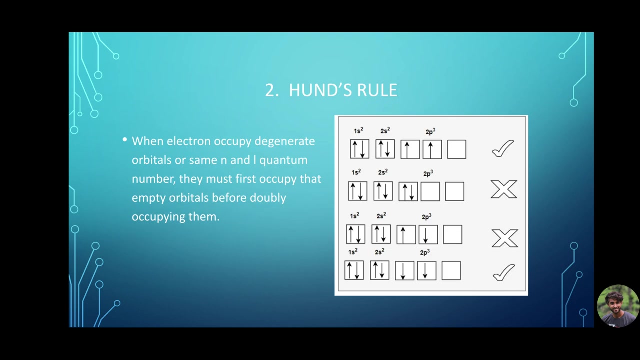 m of s ranges from minus s to plus s. An electron has spin number. s is equals to half and magnetic spin ms is equals to plus or minus half, Referring to spin up and spin down states. Now let us continue with the orbital filling rules. 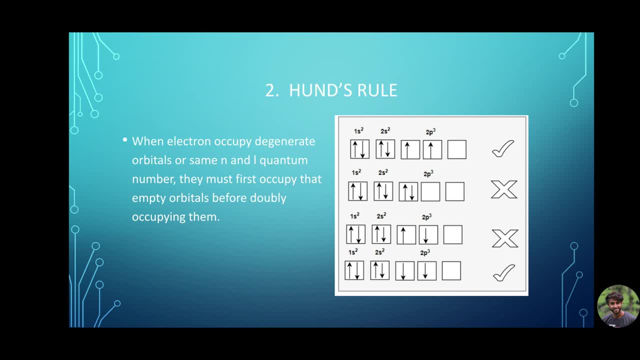 Hunt's rule. Hunt's rule states that when electron occupy degenerate orbitals or same n and l quantum numbers, they must first occupy the energy- sorry- empty orbitals before doubly occupying them. Here is an illustration. The second empty orbitals must first occupy the energy- sorry. 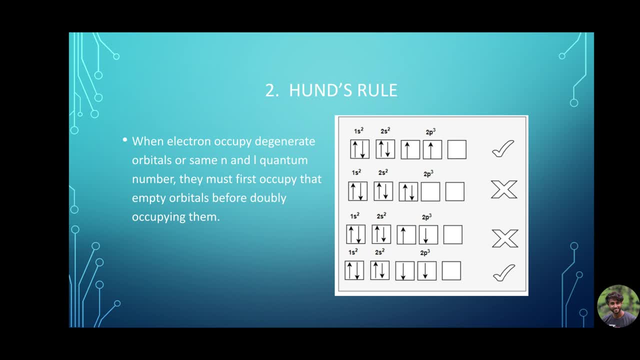 empty orbitals before doubly occupying them. Here is an illustration. The second empty orbitals must first occupy the energy- sorry, empty orbitals- before doubly occupying them. The second and third figure are not correct. The first and last figure are correct. The 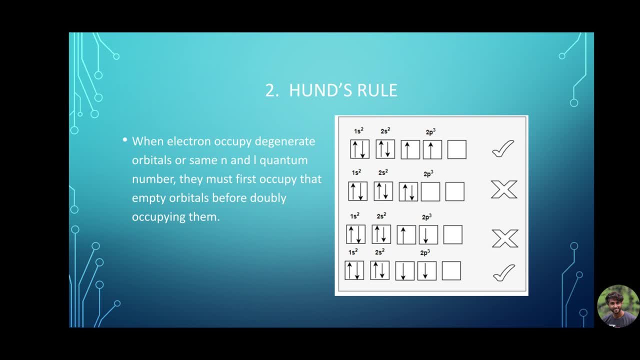 electron first is half filled, Only then are they filled. The electron first is half filled, Only then are they completely filled. Pauli Exclusion Principle. Pauli Exclusion Principle- Bio governing occurs after calibrating one item from all possible number in the entire range. 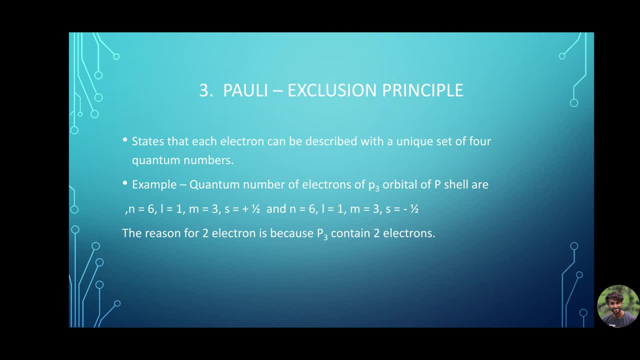 The power of positiveoxygen is Pauli exclusion principle. Pauli exclusion principle states that each electron can be described with a unique set of 4 quantum numbers. Even though 3 quantum numbers would be same, the forth quantum number should be the same amount in the näm League. 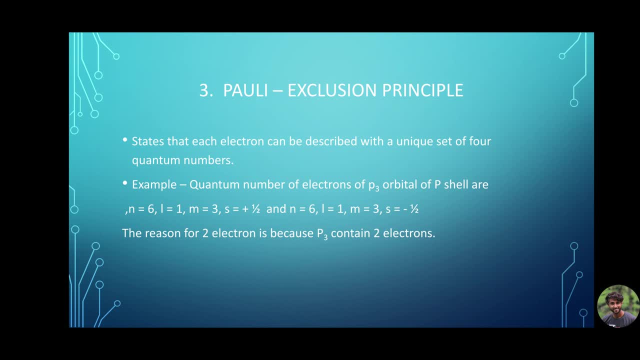 1, including the forgettable ofän tuttiác número of Self. 연иеブβ orderedходит pho accidents at the time. unknown date· the return transformed into the former number with a number notھ should be different. Thus no two electron in an atom will have four quantum numbers as same. 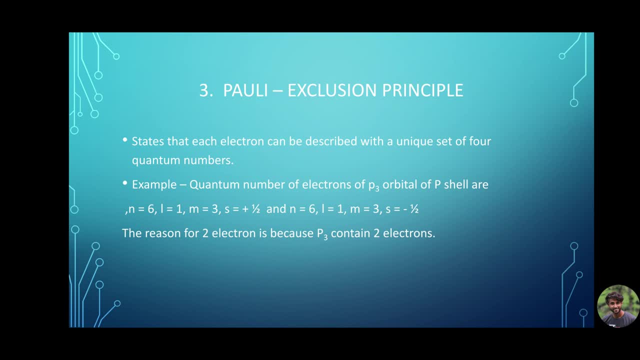 For example, an electron in the P1 orbital of the M shell has quantum number n is equals to 3, l is equals to 1, m is equals to 1 and s is equals to half and n is equals to 3,. 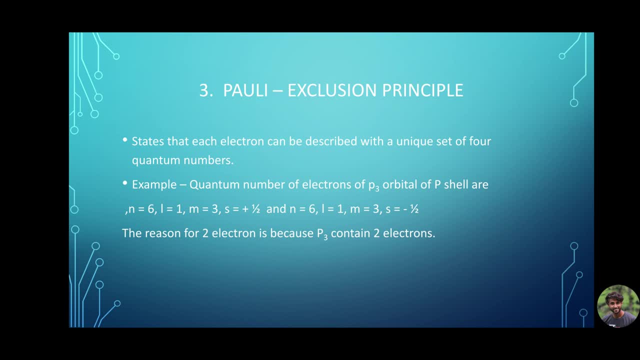 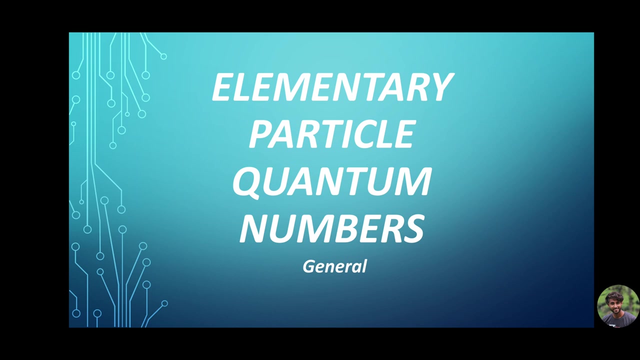 l is equals to 1, m is equals to 1 and s is equals to minus half, as there should be two electron in an orbital. Okay, now let us get down to business. Elementary Particle Quantum Number: When four previous quantum number of electron, 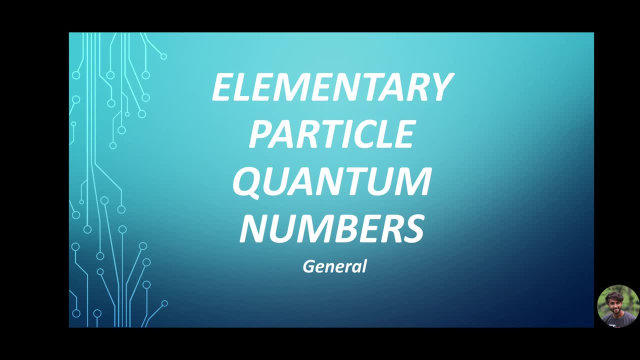 describe about an electron's position, orientation, shape, etc. to support three laws: Quantum number of elementary particles in general are a set of numerical values which describe the values of conserved quantities in a quantum system. They are characteristic variables associated with each elementary particle. 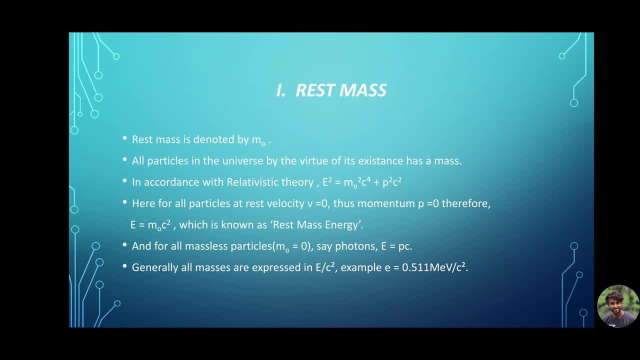 First Rest Mass. All particles in the universe, by the virtue of its existence, has a mass. It is either low or high. In particle physics, in accordance with the relativistic theory, we relate energy and mass by the general formula: E is equals to root of m0 square, c power 4 plus p square. 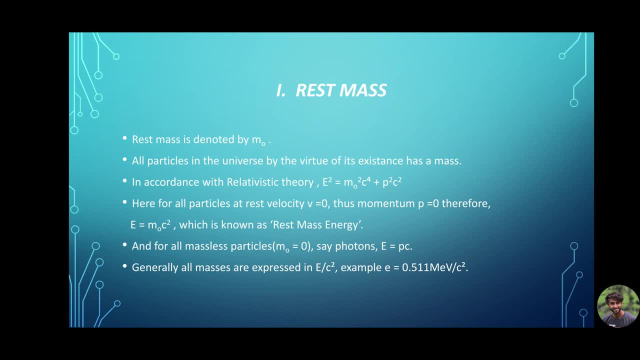 c square. For all particles that are at rest, velocity v is equals to zero. momentum p is equals to zero. Thus the formula becomes: E is equals to m0 c square. This is also known as rest energy mass. Consider photon or neutrino, for which m0 is equals to zero. 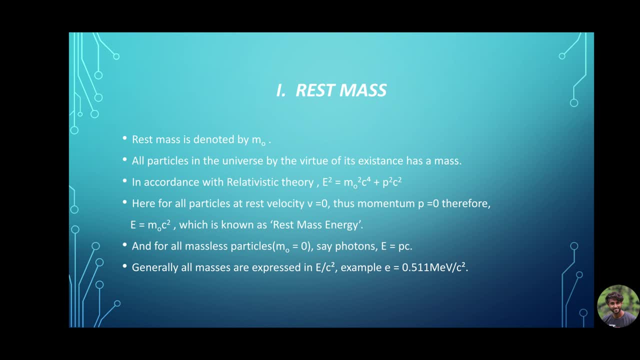 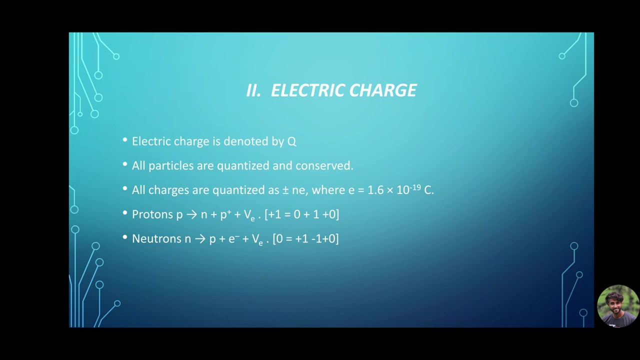 Here energy is expressed as: E is equals to p- c, But generally mass is always expressed in terms of energy by c square. For example, energy of electron E is equals to 0.511 mega electron volt by c square. Second Electric charge: All the particles which we saw in the previous. 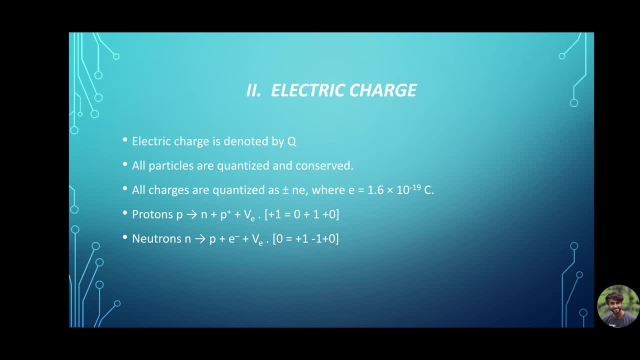 video were either positively charged, negatively charged or neutral, But irrespective of the charge, they were all quantized and conserved. This is a very, very important property. All charges are quantized: that of mass of single electron, That is plus or minus 1.6 into 10 power minus 19 coulomb. 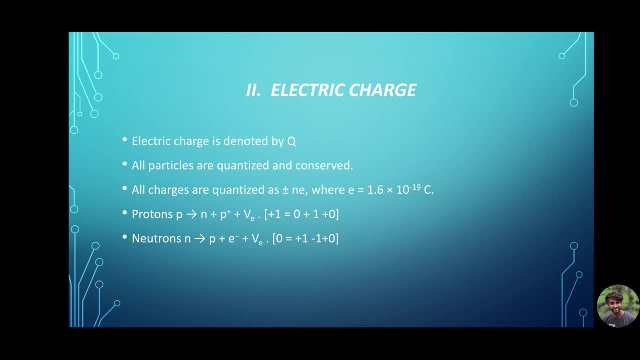 Also known as E. Thus charges will be either plus or minus Ne or zero. for neutral charge, All interaction inside the atom are conserved In beta. decay proton gives neutron positron and an anti-neutrino Proton gives neutrons. 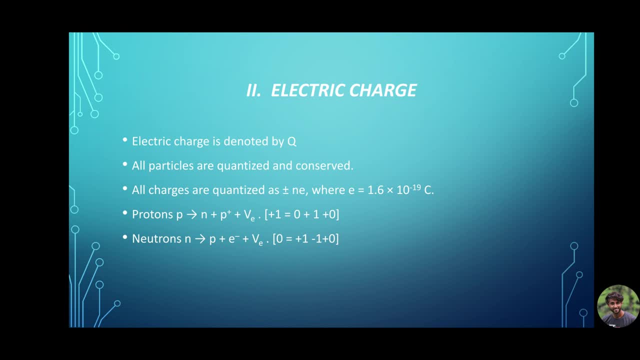 Proton gives neutrons, Neutron gives neutrons, Neutron gives neutrons. Neutron is zero or neutral, and anti-neutrino is zero. The positron is plus 1. Thus we can see that the total charge is conserved. 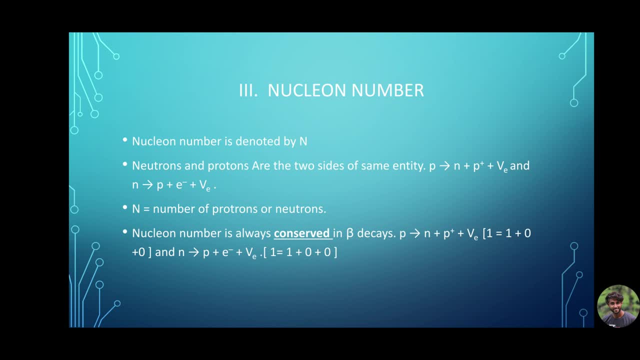 Nucleon number N. Nucleon is the combination of proton and neutron, Or in other words the constituents of nucleus. Neutron is neutral and proton is positive. It is said that neutron and proton are the two sides of the same entity. 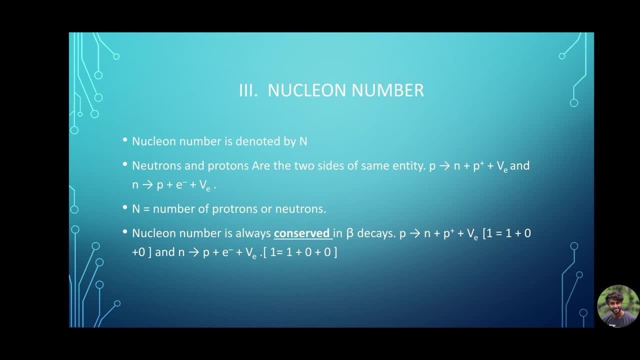 Therefore, nuclear number, capital N, is equals to number of proton or neutron. They are always conserved. Neutron decays into proton, electron and antineutrino. Nuclear number of neutron and proton is positive one, and electron and antineutrino is zero. 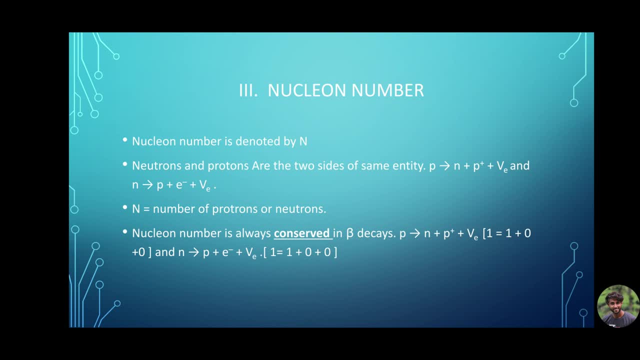 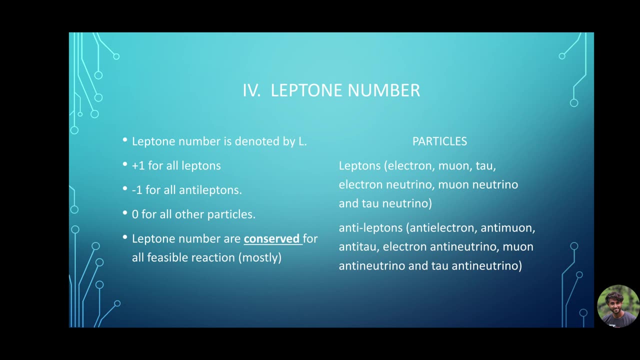 Thus the nuclear number is also conserved. Number four: lepton number, capital L. There are only three possibility for lepton number: That is positive, one, negative one or zero. For all leptons, That is Positron, muon, tau, electron, neutrino, muon, neutrino, tau neutrino. 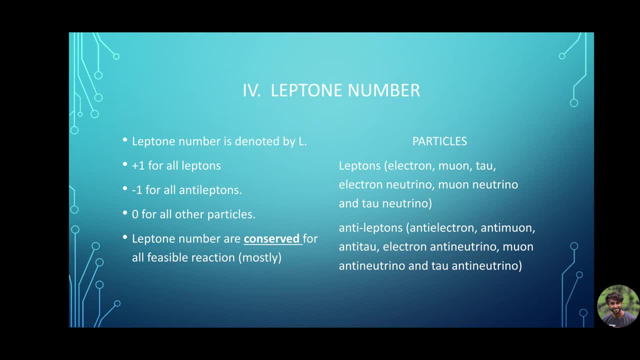 Lepton number is positive one. For all anti-lepton, That is, anti-electron or positron, anti-muon, anti-tau, electron antineutrino, muon antineutrino and tau antineutrino, Lepton number is negative one. 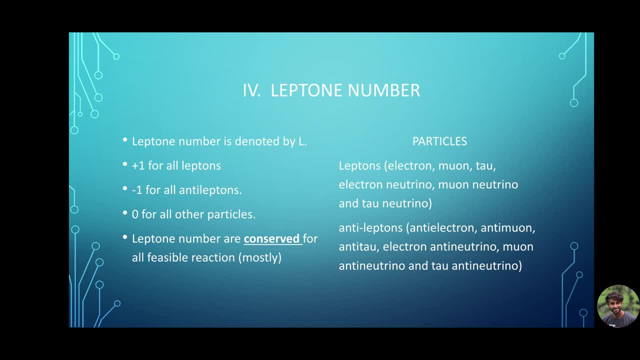 And finally, for all other particle, lepton number is zero. In order for all processes to be feasible, lepton number should be conserved. Fifth baryon number: If you remember from the previous videos, baryon was made up of odd number of valence. 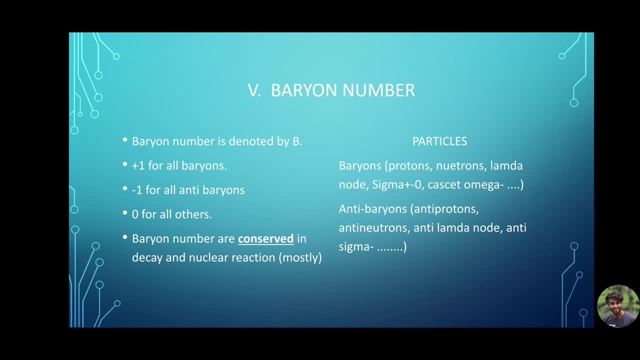 quark, Similar to lepton number. baryon number can be positive one, negative one or positive one And finally, for all other particle, lepton number is zero. In order for all processes to be feasible, lepton number should be conserved. In order for all processes to be feasible, lepton number should be conserved And, finally, for all other particles to be feasible, baryon number should be conserved. Similar to lepton number, baryon number can be positive one, negative one or positive. 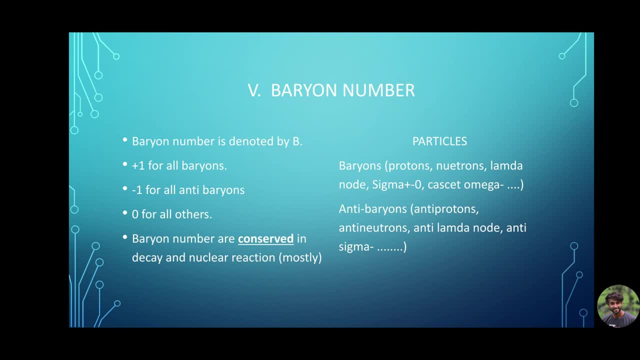 one Positive one: when we have baryon, That is proton, neutron, lambda, not sigma minus, sigma plus sigma zero, casket, omega minus, etc. Baryon number is negative one. when we have an antibaryon, 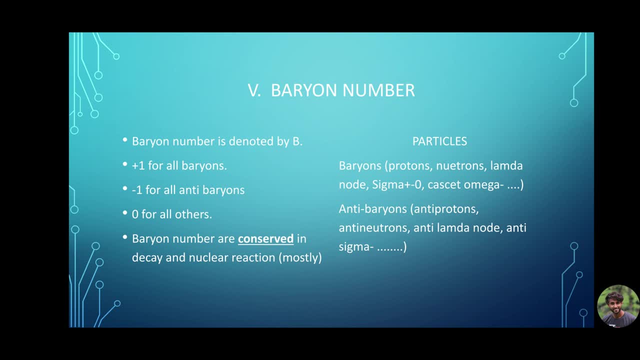 That is, antiproton, antineutron, antilambdax, lambda naught, anti-sigma minus, etc. and zero when none of these. If you want to know more about baryon, click on the right top corner. Now baryon number is always conserved in decay processes and nuclear action. 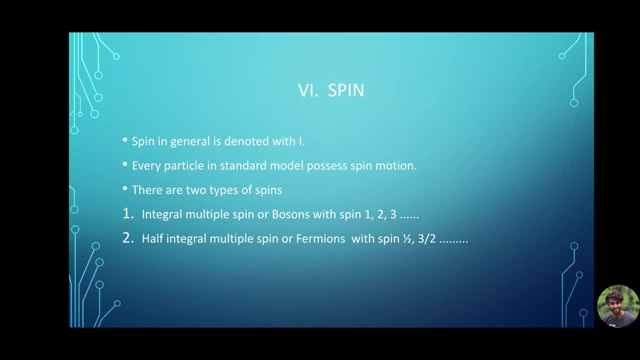 Sixth spin quantum number, capital I. It is observed that all elementary particle possesses spin motion, and this spin is classified into two parts: Number one, particle which spin in integral multiples, or also known as boson, and second, particles which spin in half integrals, multiple or fermions. 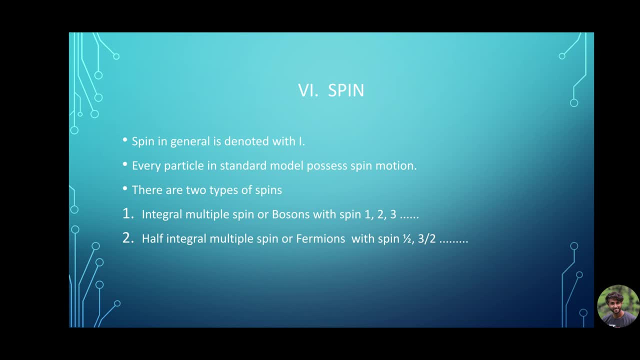 In previous video we have discussed about what fermion and bosons are. If you haven't watched that video, click on the right top corner, If you notice. this is the same quantum number in the electron. The reason for its half spin is because of being a lepton in fermions.